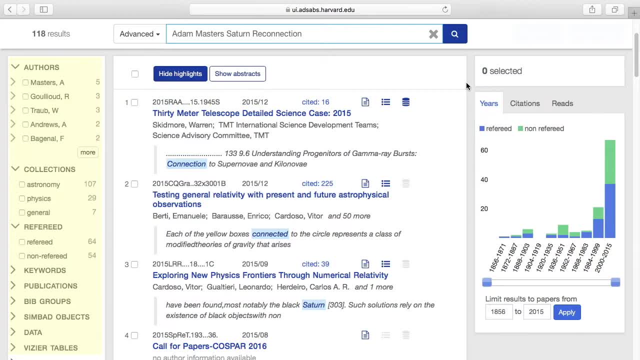 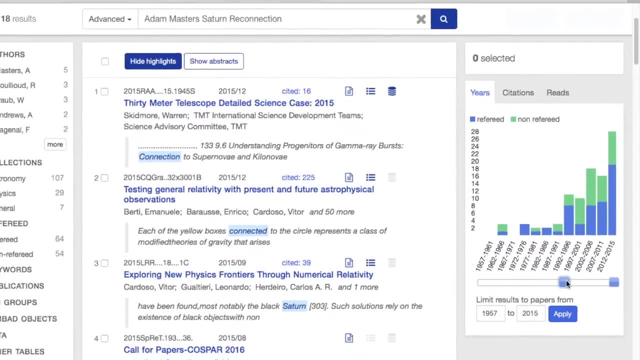 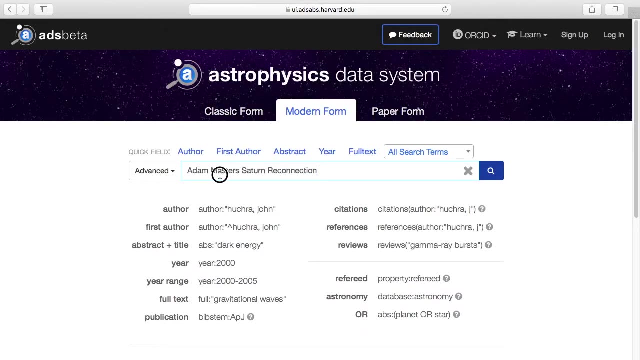 You can narrow down the results by using the filters. For example, you can limit the results to papers published in a certain date range. Let's go back to the search page and carry out a more targeted inquiry using search fields. You can build a fielded search inquiry using search fields like author or title. 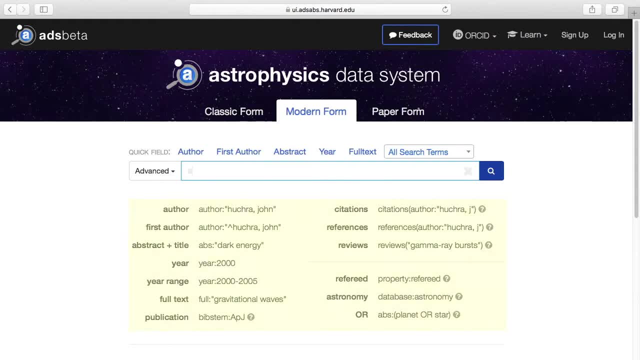 Examples of the most commonly used search fields are on the main search page. For example, by setting the search fields for author to Masters, Adam, title to Saturn and abs- meaning abstract to reconnection, This means ADS will search for articles with the first author, Adam Masters, with the title containing 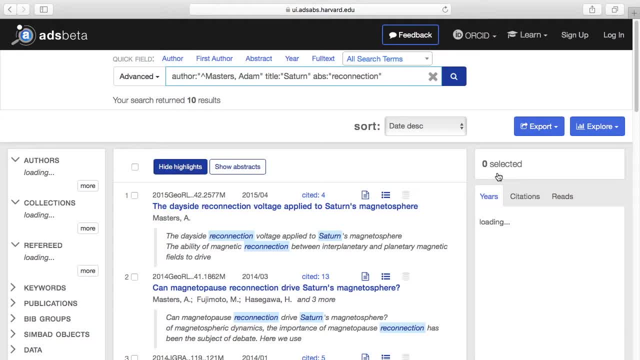 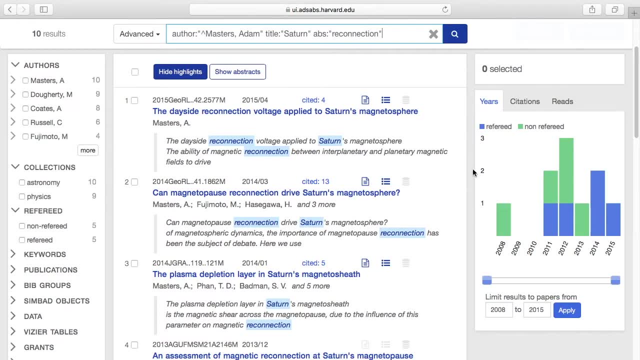 Saturn and the abstract containing Reconnection. There are only 10 results. now Let's talk about the results. On the results page, a list of the articles is displayed in the middle, with the titles, authors and a relevant excerpt from the text. 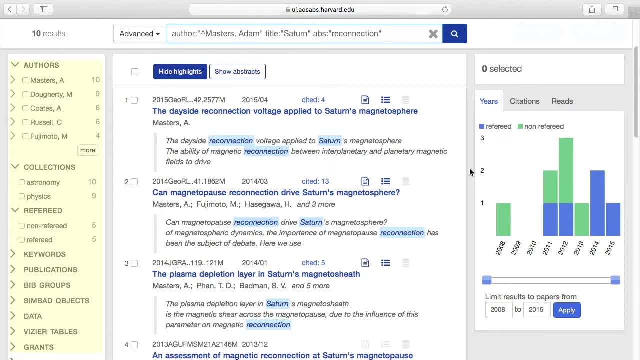 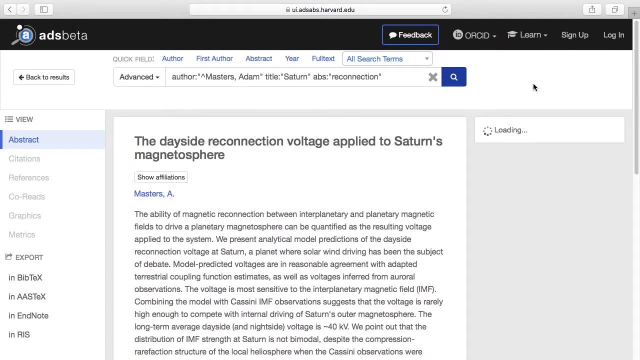 On the left, several different filter functions are available, such as author and keywords. At the top, various sorting functions are available. Let's look at a single article by clicking on one of the titles. Here the title and abstract of the article can be seen, along with other useful information about the article. 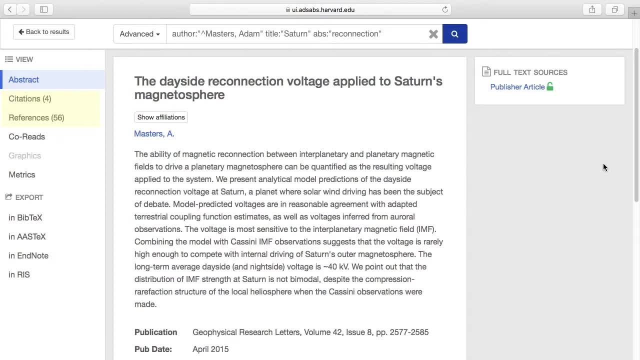 On the left. the citations of the article can be seen under Citations, and papers referenced by the article are under References. Below that, several methods of exporting the bibliographic reference can be seen, including BibTeX, Aztek and EndNote. 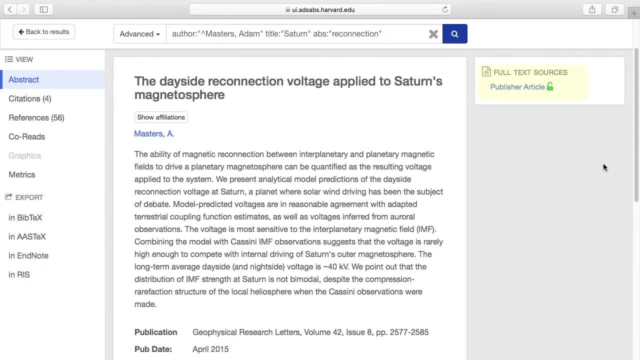 Finally, on the right, there will be a link where you can download the full text of the published article or, if available, the archive ePrint. Please note that you will only be able to download the full text of the published article. You can download recent published articles if they are open access or if you or your library subscribe to the journal.